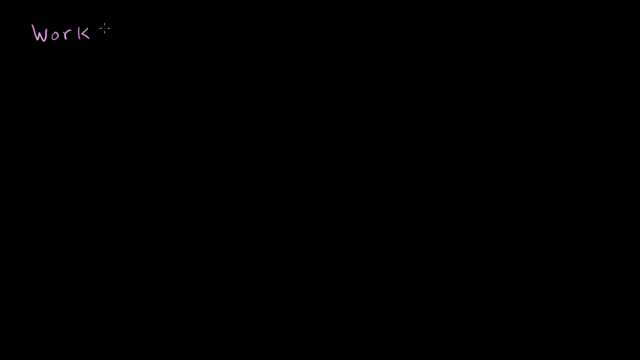 the same direction as your displacement. So you learn that work is really the magnitude of the force in the direction, or the component of the force in the direction in direction of a displacement. Displacement is just distance with some direction In direction of displacement times the magnitude of 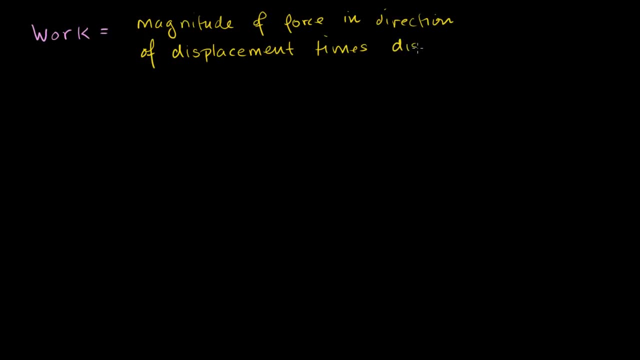 the displacement. Or you could just kind of say: times the distance, displaced, Times the distance. I'm not being too particular about it. And the classic example: maybe you have an ice cube or some type of block. I just say ice, so that it's not a lot of friction. 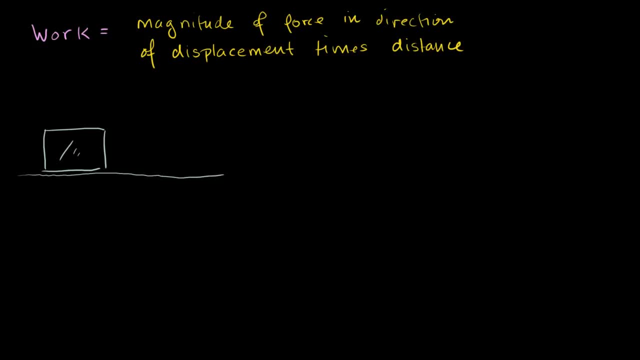 Maybe it's standing on a bigger sheet of lake or ice of something And maybe you're pulling on that ice cube at an angle. Let's say: you're pulling at an angle like that, That is my force right there. Let's say: my force is equal to. 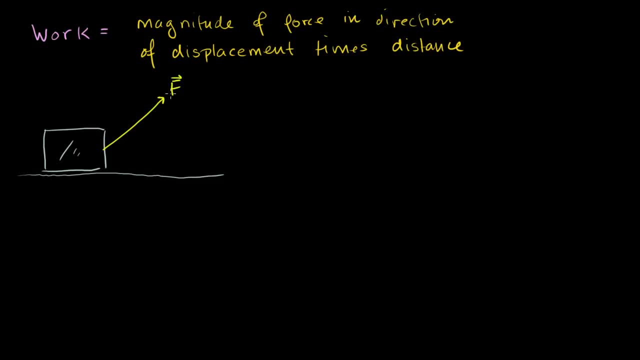 Well, that's my force vector, Let's say the magnitude of my force vector. So I'll say the magnitude. So I'm going to put two brackets around there. The magnitude of my force vector we can say is, let's say it's 10 Newtons. 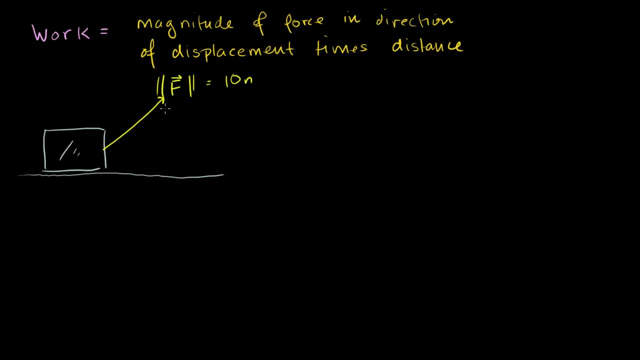 And let's say the direction of my force vector. Any vector has to have a magnitude and a direction. And the direction- let's say it has a 30 degree angle, Let's say it's 60 degree angle above horizontal. So that's the direction I'm pulling in. 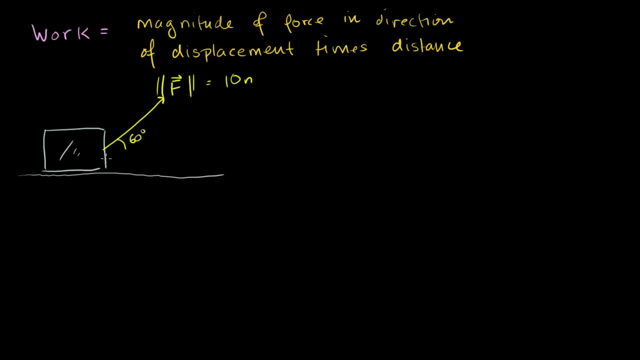 And let's say I displace it. This is all a bit of review, hopefully, If you're displacing it, let's say you displace it 5 Newtons, So let's say the displacement, That's the displacement vector, right there. 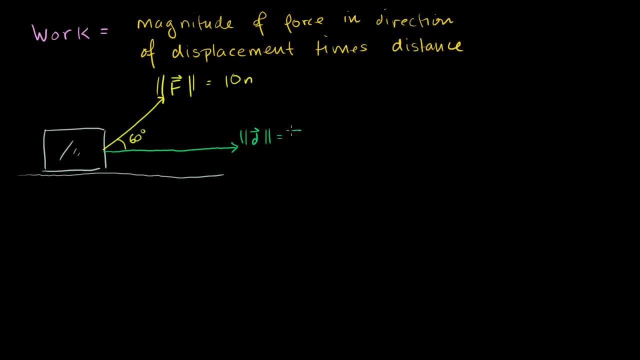 And the magnitude of it is equal to 5 meters. So you've learned from the definition of work. You can't just say, oh, I'm pulling with 10 Newtons of force and I'm moving it 5 meters. You can't just multiply the 10 Newtons times the 5 meters. 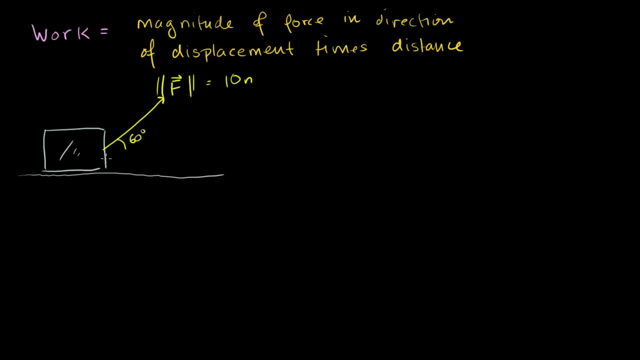 And let's say I displace it. This is all a bit of review. hopefully, If you're displacing it, let's say you displace it 5 newtons, So let's say the displacement, That's the displacement vector right there. 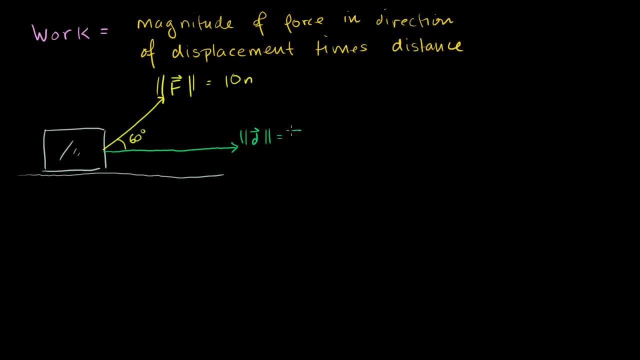 And the magnitude of it is equal to 5 meters. So you've learned from the definition of work. You can't just say, oh, I'm pulling with 10 newtons of force and I'm moving it 5 meters. You can't just multiply the 10 newtons times the 5 meters. 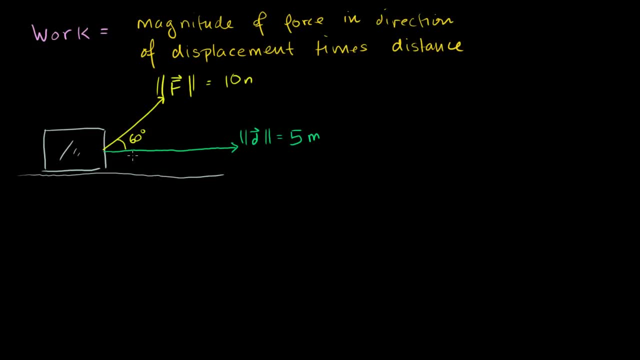 You have to find the magnitude of the component going in the same direction as my displacement. So what I essentially need to do is, if you imagine the length of this vector being 10, that's the total force, But you need to figure out the length of the vector, that's. 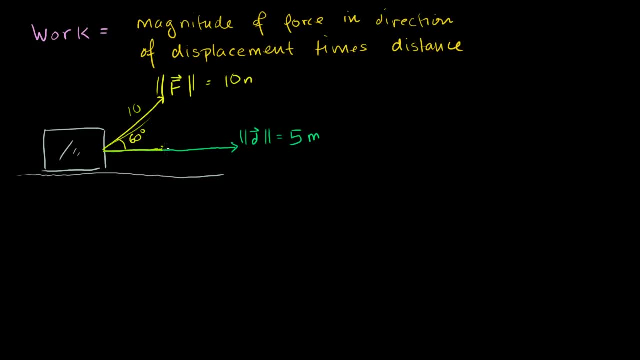 the component of the force going in the same direction as my displacement, And a little simple trigonometry. You know that this is 10 times the cosine of 60 degrees, Or that's equal to cosine of 60 degrees is 1 half. 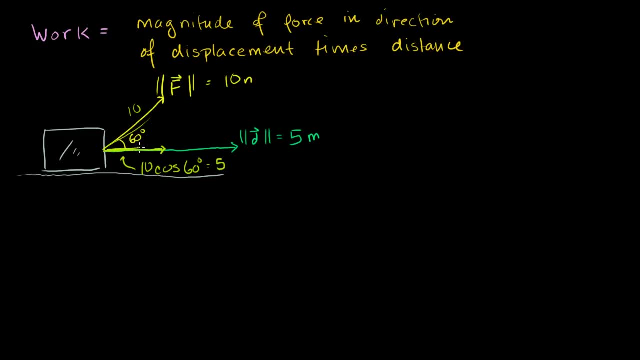 So that's just equal to 5.. So this magnitude, the magnitude of the force going in the same direction of the displacement, in this case, is 5 newtons, And then you can figure out the work. You could say that the work is equal to 5 newtons times. 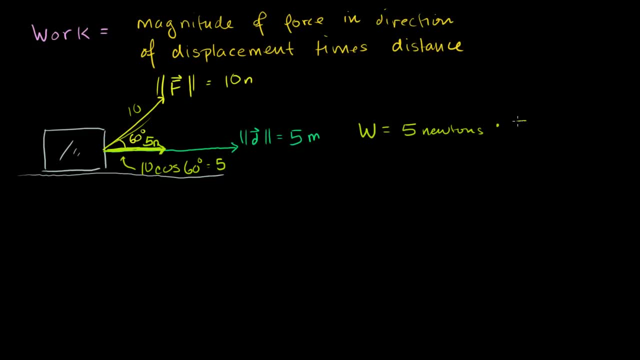 Well, I'll just write a dot for times. I don't want you to think it's cross product Times: 5 meters, which is 25 newton meters, Or you could even say 25 joules of work have been done. 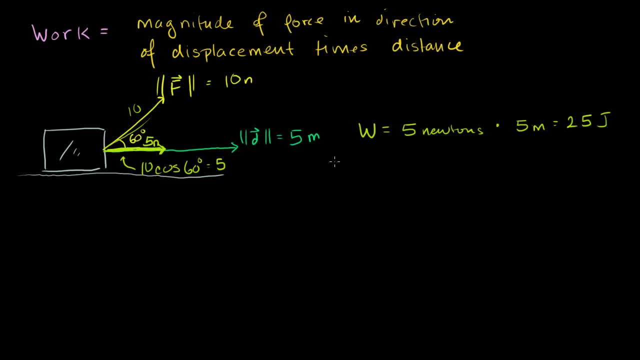 And this is all really a review of somewhat basic physics. But just think about what happened here. What was the work? If I write it in the abstract, the work is equal to the 5 newtons. that was the magnitude of my force vector. 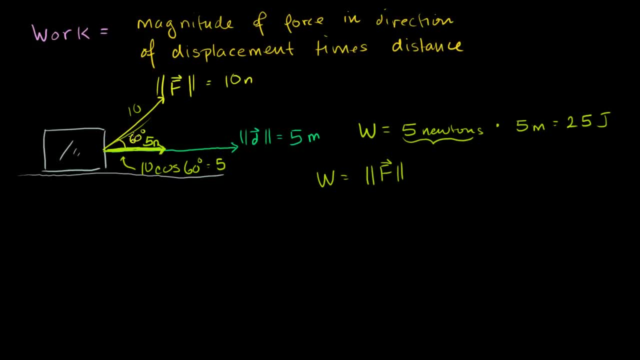 So it's the magnitude of my force vector times the cosine of this angle. Times the cosine- So let's call that theta, Let's say it a little generally- So- times the cosine of the angle, This is the amount of my force in the direction of the. 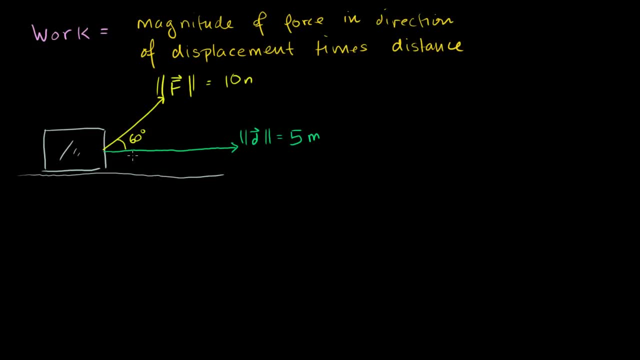 You have to find the magnitude of the component going in the same direction as my displacement. So what I essentially need to do is, if you imagine the length of this vector being 10, that's the total force, But you need to figure out the length of the vector, that's. 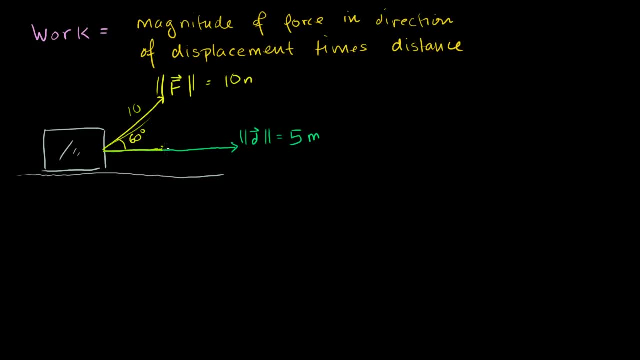 the component of the force going in the same direction as my displacement, And a little simple trigonometry. You know that this is 10 times the cosine of 60 degrees, Or that's equal to cosine of 60 degrees is 1 half. 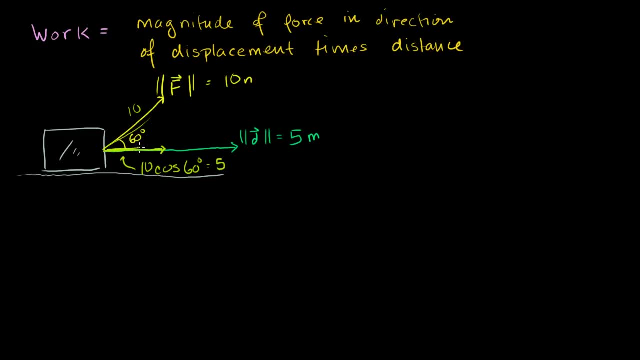 So that's just equal to 5.. So this magnitude, the magnitude of the force going in the same direction of the displacement, in this case, is 5 Newtons, And then you can figure out the work. You could say that the work is equal to 5 Newtons times. 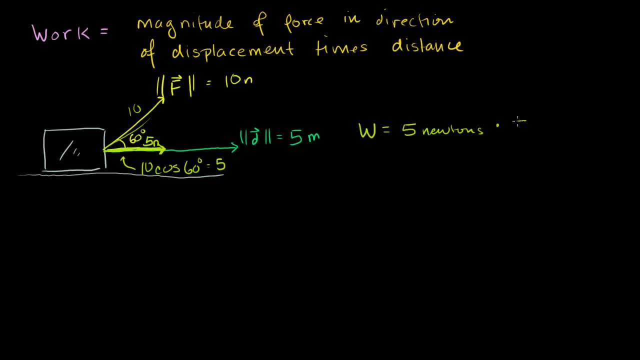 Well, I'll just write a dot for times- I don't want you to think it's cross product Times- 5 meters, which is 25 Newton meters, Or you could even say 25 Joules of work have been done, And this is all really a review of somewhat basic physics. 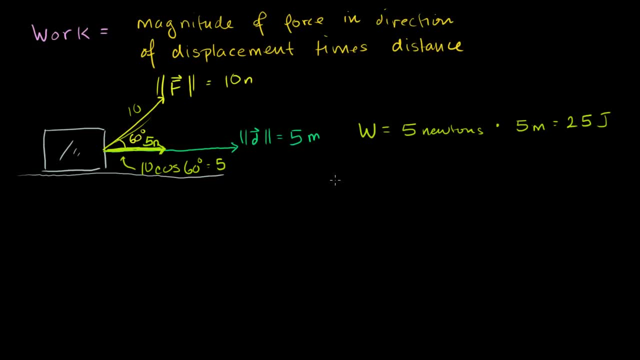 But just think about what happened here. What was the work? If I write it in the abstract, the work is equal to the 5 Newtons- that was the magnitude of my force vector- times the cosine of this angle. So let's call that theta. 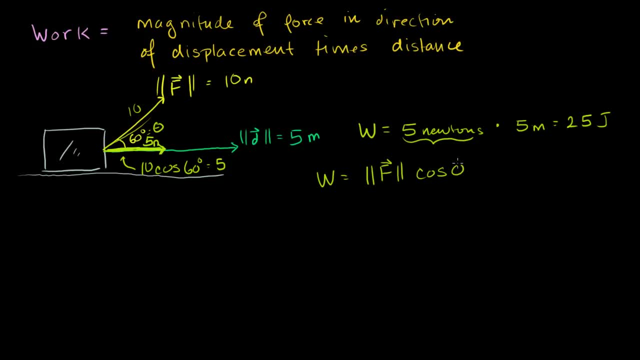 Let's say it a little generally. So times the cosine of the angle. This is the amount of my force in the direction of the displacement. the cosine of the angle between them times the magnitude of the displacement. Or if I wanted to rewrite that, I could just write that as the 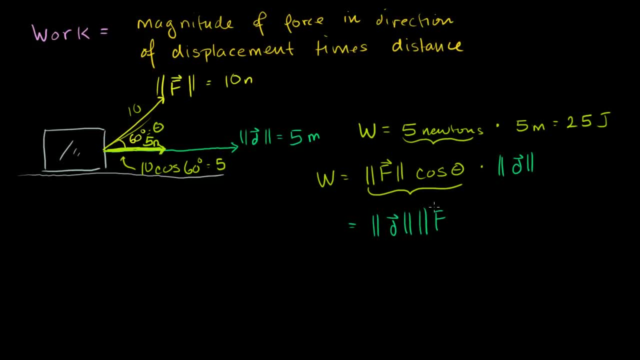 magnitude of the displacement times, the magnitude of the force Times the cosine. Let's say this is a fraction of the theta And I've done multiple videos of this in the linear algebra playlist, in the physics playlist where I talk about the dot product and the cross product and all of that. 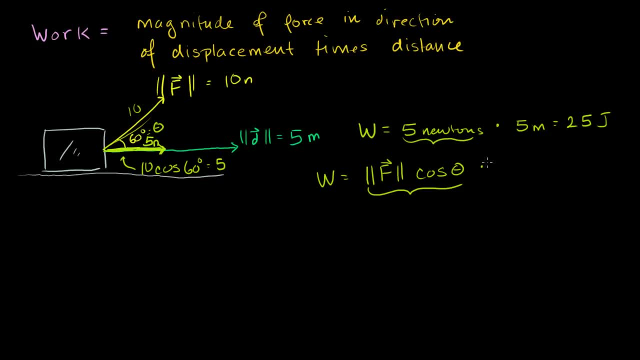 displacement. the cosine of the angle between them times the magnitude of the displacement. Or if I wanted to rewrite that, I could just write that as the magnitude of the displacement times the magnitude of the force times the cosine, So the cosine of theta. 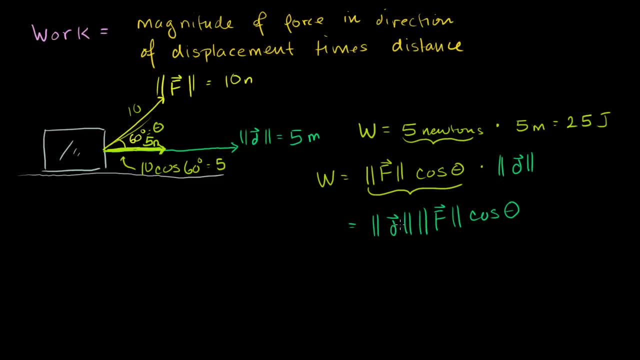 And I've done multiple videos of this in the linear algebra playlist, in the physics playlist, where I talk about the dot product and the cross product and all of that. But this is the dot product of d and f, of the vectors d and f. 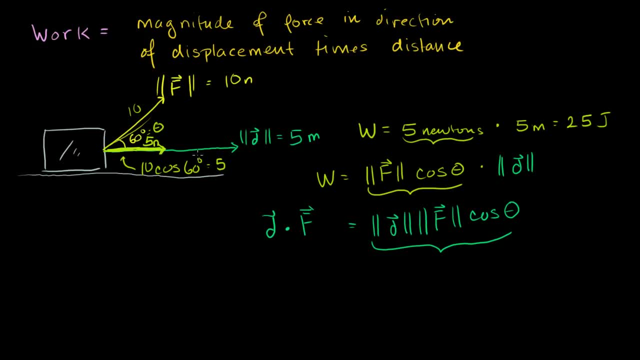 So, in general, if you're trying to find the work for a constant displacement and you have a constant force, you just take the dot product of those two vectors And if the dot product is a completely foreign concept, you might want to watch it. 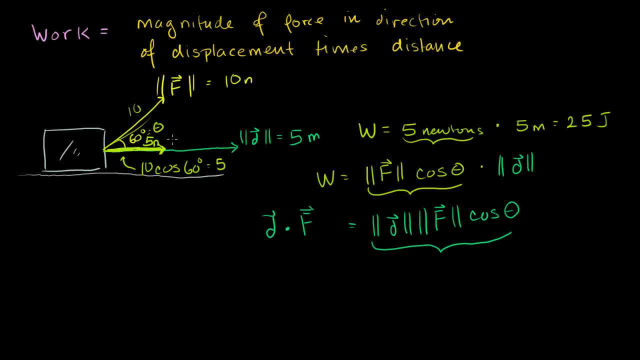 There's another one in the class, I'm not going to go through all of them watched. I think I've made multiple four or five videos on the dot product and its intuition and how it compares, But just to give you a little bit of that intuition, right. 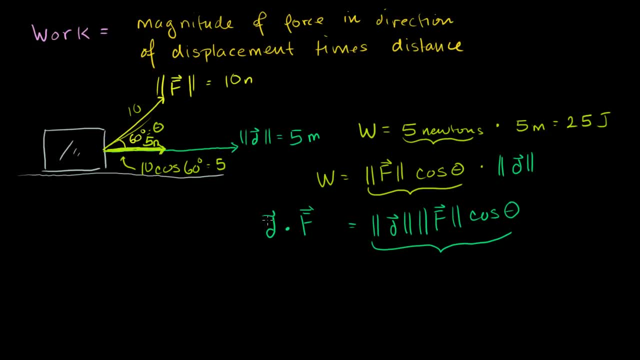 here, the dot product. when I take f dot d or d dot f, what it's giving me is: I'm multiplying the magnitude. Well, I could just read this out. but the idea of the dot product is: take how much of this vector is going in the 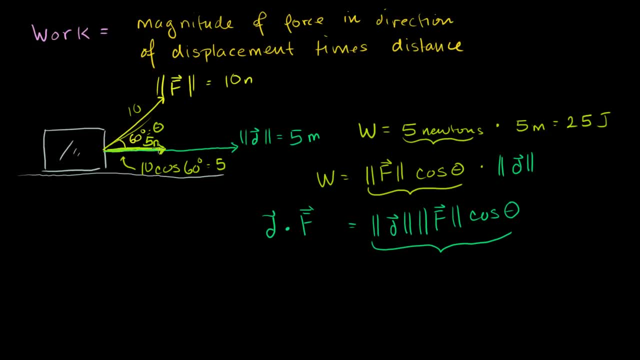 same direction as this vector, and in this case it's this much, and then multiply the two magnitudes And that's what we did right here. So the work is going to be the force vector, dot, taking the dot product of the force vector with the displacement. 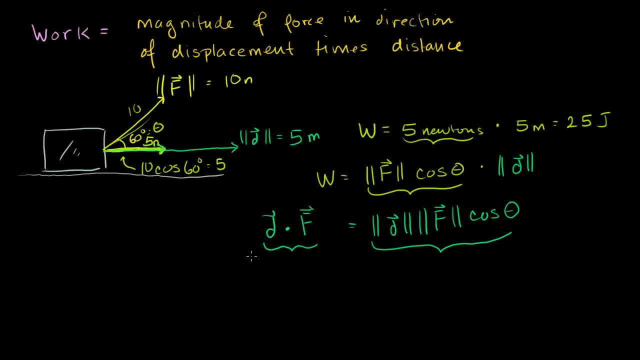 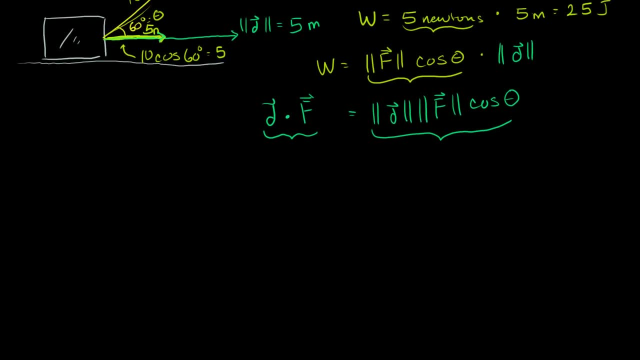 vector, and this, of course, is a scalar value, And we'll work out some examples in the future where you'll see that that's true. So this is all a review of fairly elementary physics. Now let's take a more complex example, but it's. 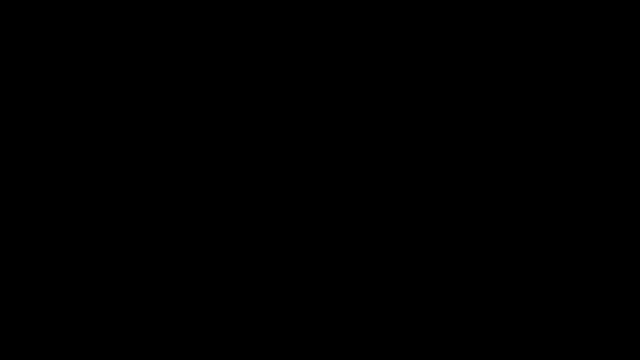 really the same idea. Let's define a vector field. So let's say that I have a vector field f, And we're going to think about what this means in a second. It's a function of x and y and it's equal to some scalar. 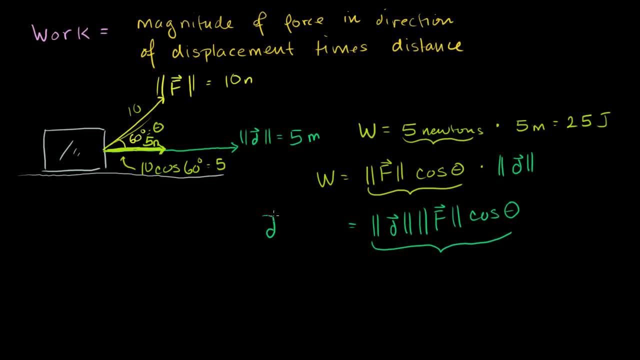 But this is the dot product of d and f, of the vectors d and f. So in general, if you're trying to find the work for constant displacement and you have a constant force, you just take the dot product of those two vectors. 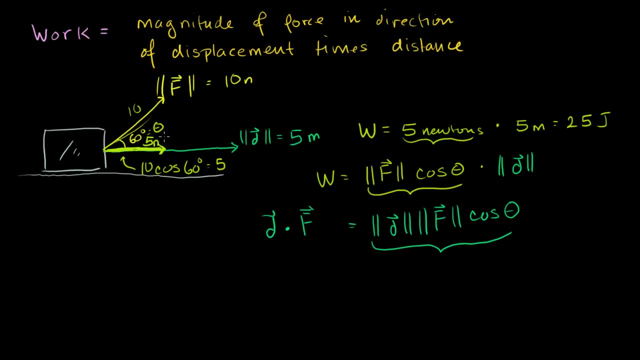 And if the dot product is a completely foreign concept to you, you might want to watch that. I think I've made multiple- four or five- videos on the dot product and its intuition and how it compares, But just to give you a little bit of that intuition, right. 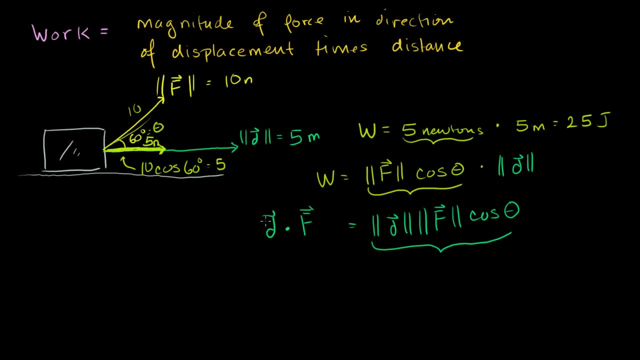 here, the dot product. when I take f dot d or d dot f, what it's giving me is: I'm multiplying the magnitude. Well, I could just read this out. but the idea of the dot product is: take how much of this vector is going in the 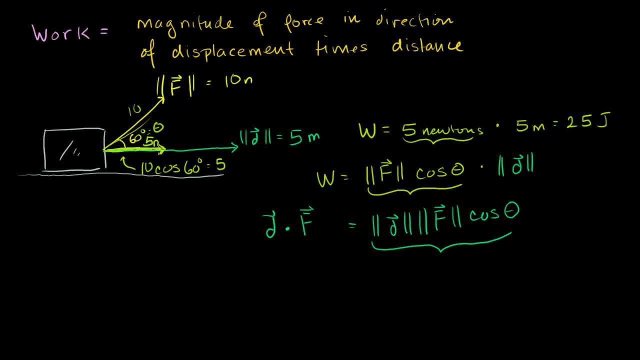 same direction as this vector, and in this case it's this much, and then multiply the two magnitudes And that's what we did right here. So the work is going to be the force vector, dot, taking the dot product of the force vector with the displacement. 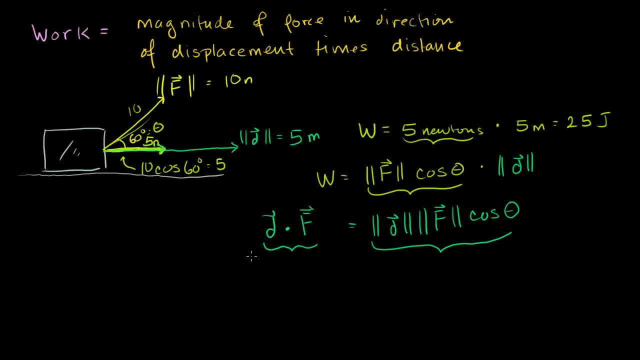 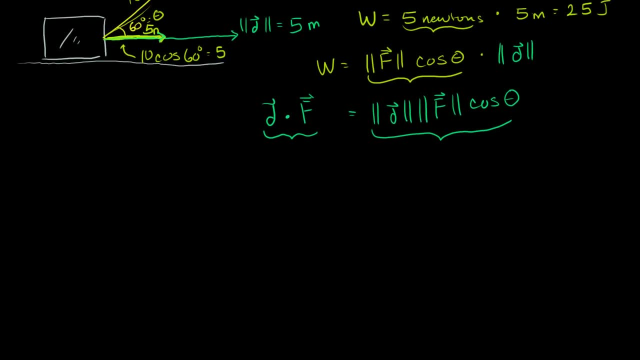 vector, and this, of course, is a scalar value, And we'll work out some examples in the future where you'll see that that's true. So this is all a review of fairly elementary physics. Now let's take a more complex example, but it's. 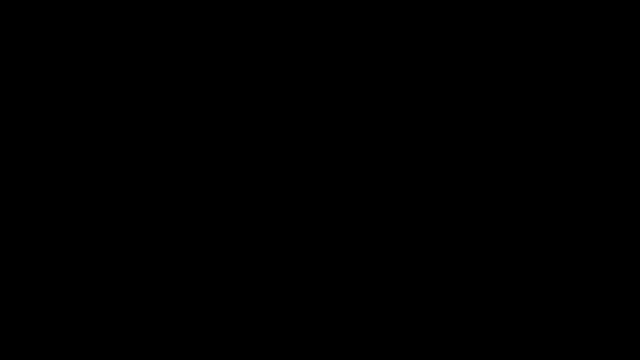 really the same idea. Let's define a vector field. So let's say that I have a vector field f, And we're going to think about what this means in a second. It's a function of x and y and it's equal to some scalar. 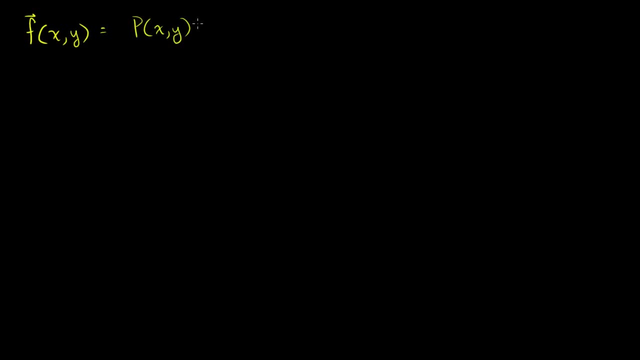 function of x and y times the i unit vector or the horizontal unit vector plus some other function: scalar function of x and y times the vertical unit vector. So what would something like this be? This is a vector field. This is a vector field in two-dimensional space or on. 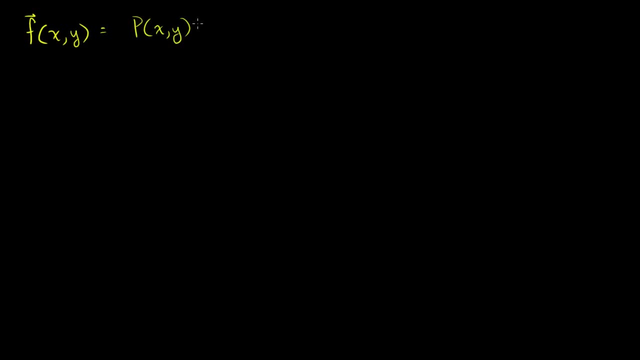 function of x and y times the i unit vector or the horizontal unit vector plus some other function: scalar function of x and y times the vertical unit vector. So what would something like this be? This is a vector field. This is a vector field in two-dimensional space or on. 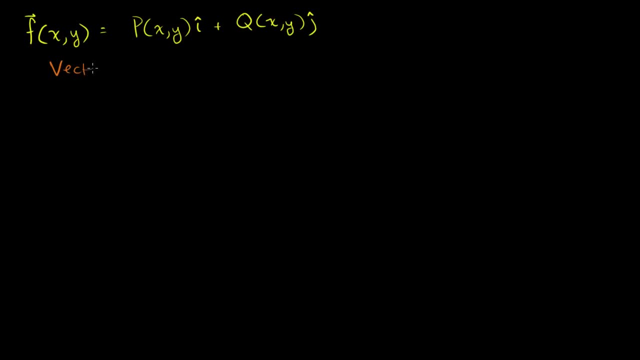 the xy-plane. This is a vector field on xy-plane, Or you could even say on or on R2.. Either way, I don't want to get too much into the mathiness of it, but what does this do? Well, if I were to draw my xy-plane, so that is my. 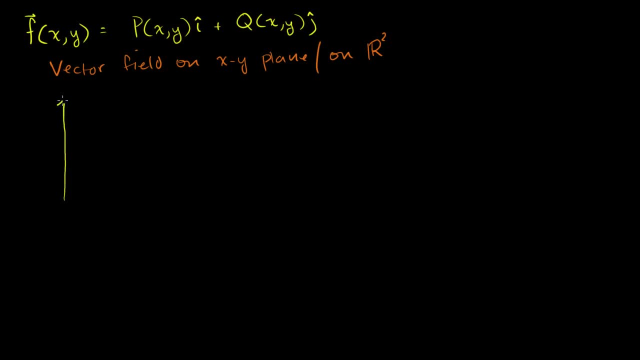 again, I'm having trouble drawing a straight line. All right, there we go. That's my y-axis and that's my x-axis. I'm just drawing the first quadrant, but you could go negative in either direction if you like. 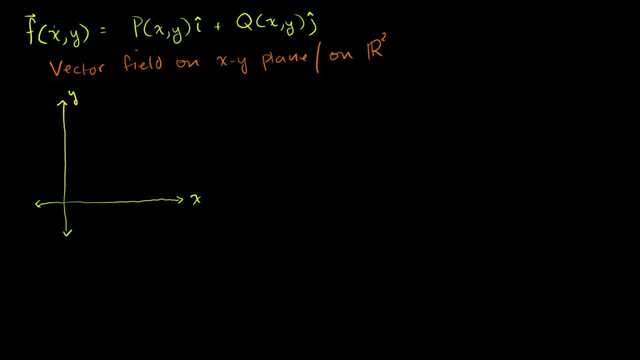 What does this thing do? Well, it's essentially saying: look, you give me any x, any y, You give any xy in the xy-plane, and these are going to end up with some numbers. right, When you put xy here, you're going to get some value and 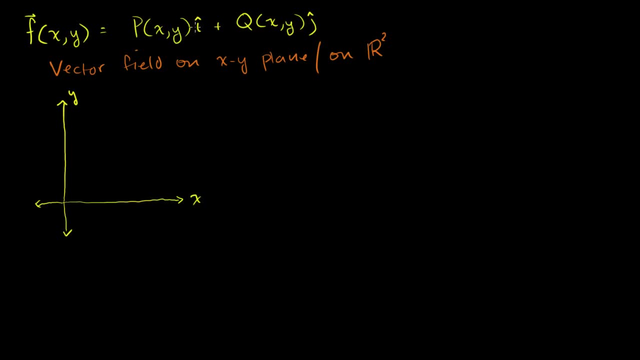 when you put xy here, you're going to get some value, So you're going to get some combination of the i and j unit vector, So you're going to get some vector. So what this does is it does this. It defines a vector that's associated with every point on. 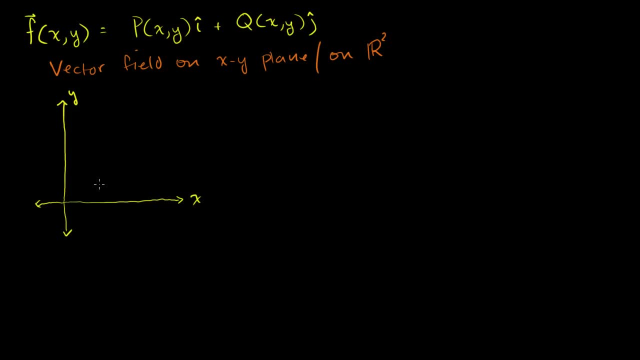 the xy-plane. So you could take. you could say, hey, if I take this point on the xy-plane and I were to pop it into this, I'll get something times i plus something times j, and when you add those two maybe I get a vector that looks like. 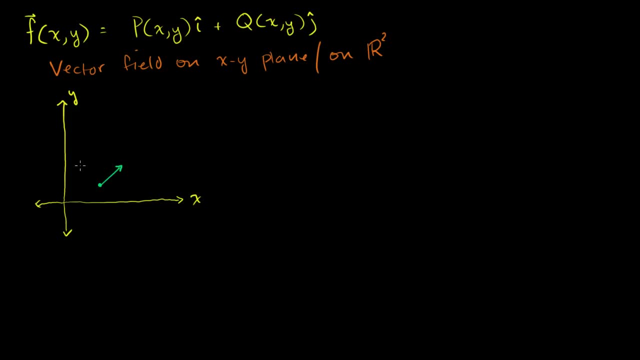 something like that, And you can do it on every point. I'm just taking random samples. Maybe when I go here, the vector looks something like that. Maybe when I go here, the vector looks like this. Maybe when I go here, the vector looks like that. 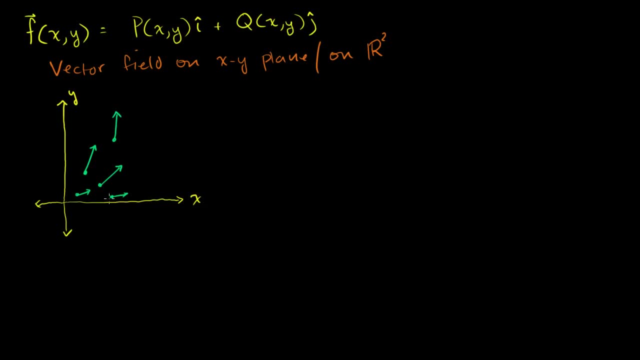 Maybe when I go up here the vector goes like that- I'm just randomly picking points. It defines a vector on all of the xy-coordinates where these functions, these scalar functions, are properly defined, and that's why it's called a vector field. 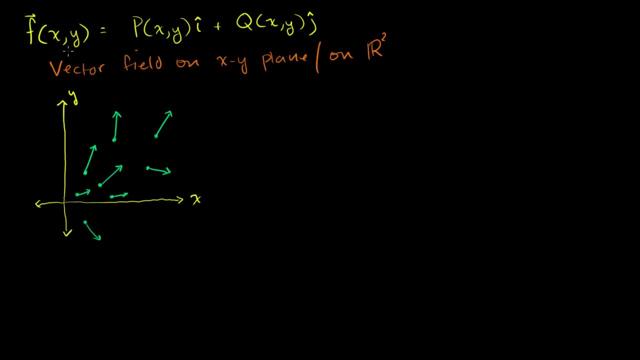 It defines what a potential maybe force would be or some other type of well, we could say force at any point. If you happen to have something there, maybe that's what the function is, And I could keep doing this forever and 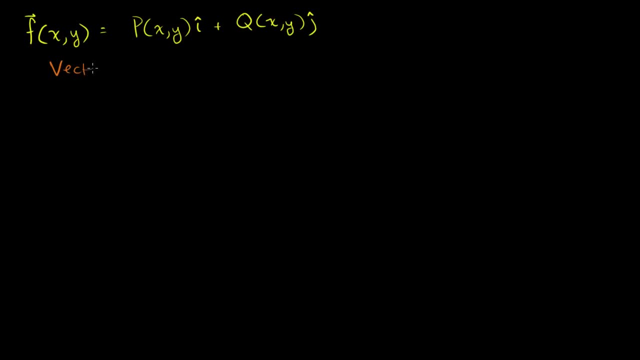 the xy-plane. This is a vector field on xy-plane, Or you could even say on or on R2.. Either way, I don't want to get too much into the mathiness of it, but what does this do? Well, if I were to draw my xy-plane, so that is my. 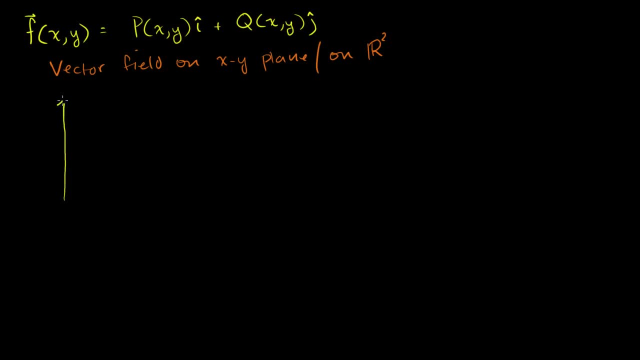 again, I'm having trouble drawing a straight line. All right, there we go. That's my y-axis and that's my x-axis. I'm just drawing the first quadrant, but you could go negative in either direction if you like. 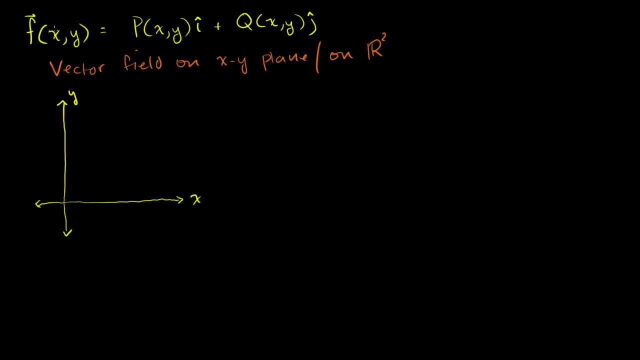 What does this thing do? Well, it's essentially saying: look, you give me any x, any y, You give any xy in the xy-plane, and these are going to end up with some numbers. right, When you put xy here, you're going to get some value. 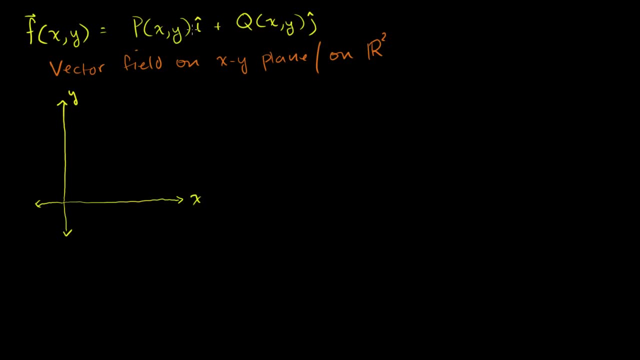 And when you put xy here, you're going to get some value. So you're going to get some combination of the i and j unit vector, So you're going to get some vector. So what this does is: it does this, It does this. 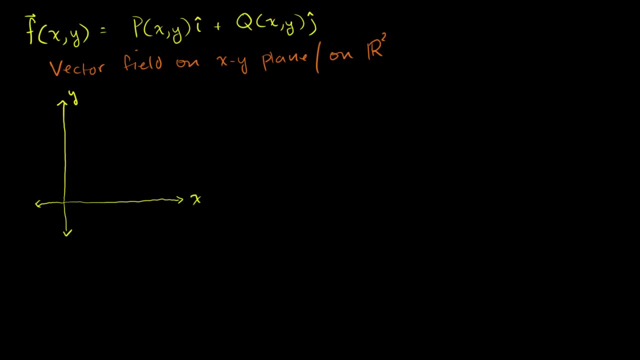 It defines a vector that's associated with every point on the xy-plane. So you could say, hey, if I take this point on the xy-plane and I were to pop it into this, I'll get something times i plus something times j. 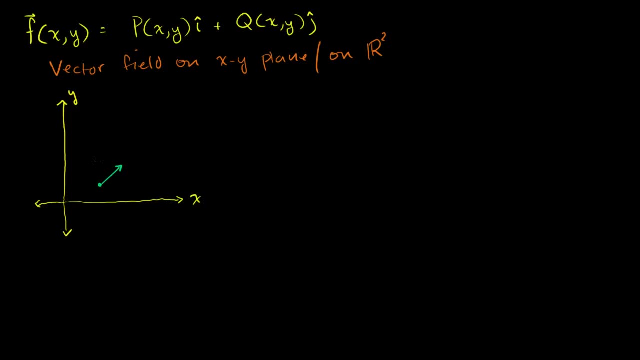 And when you add those two, maybe I get a vector that looks like something like that And you can do it on every point. I'm just taking random samples. Maybe when I go here the vector looks something like that. Maybe when I go here, the vector looks like this. 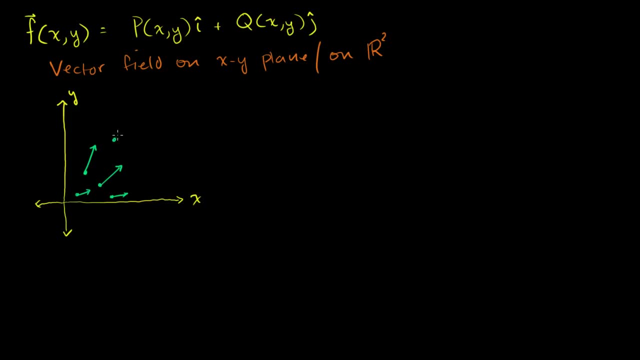 Maybe when I go here the vector looks like that. Maybe when I go up here the vector goes like that. I'm just randomly picking points. It defines a vector on all of the xy-coordinates where these scalar functions are properly defined. 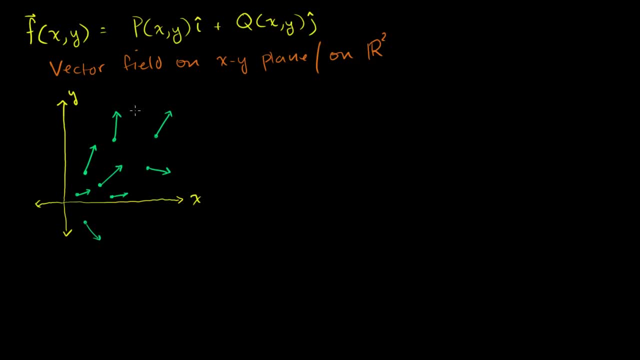 And that's why it's called a vector field. It defines what a potential maybe force would be or some other type of well we could say force at any point, If you happen to have something there, maybe that's. 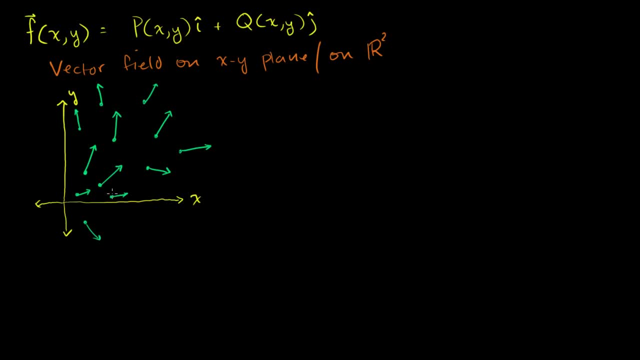 what the function is, And I could keep doing this forever and filling in all the gaps, but I think you get the idea. It differentiates a vector with every point on the xy-plane. Now this is called a vector field, so it probably makes a. 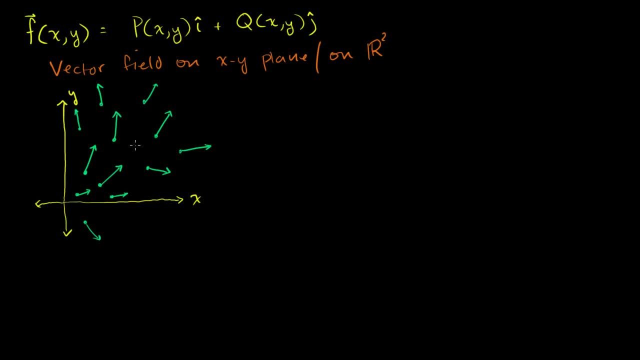 filling in all the gaps, But I think you get the idea. It associates a vector with every point on the xy-plane. Now this is called a vector field, so it probably makes a lot of sense that this could be used to describe any type of 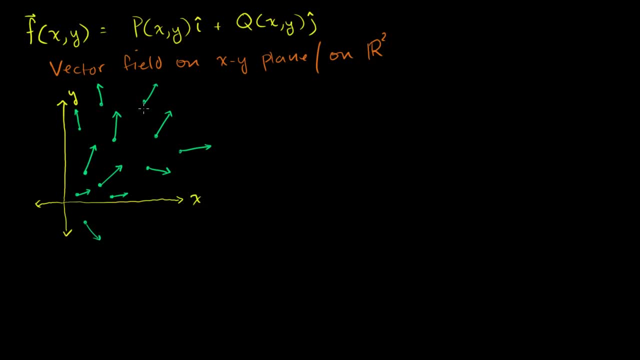 field. It could be a gravitation field, It could be an electric field, It could be a magnetic field, And this could be essentially telling you how much force there would be on some particle in that field. That's exactly what this would describe. 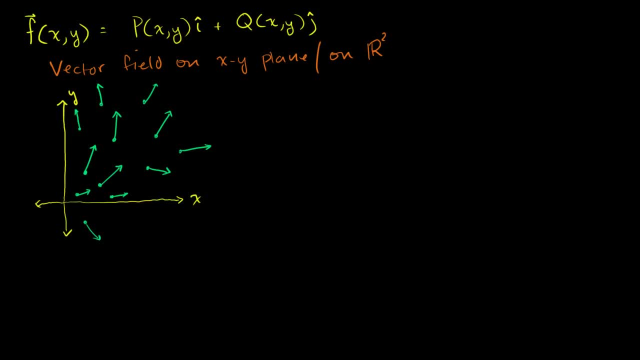 Now let's say that in this field, I have some particle traveling on the xy-plane And let's say it starts here, Let's say it starts there And by virtue of all of these crazy forces that are acting on it- and maybe it's on some tracks or something- 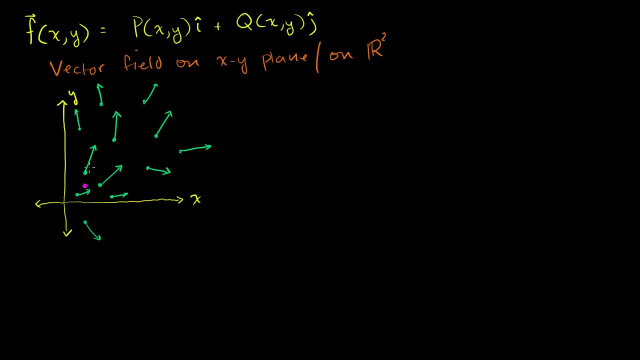 So it won't always move exactly in the direction that the field is trying to move it at. So let's say it moves in a path that moves something like this, And let's say that this path or this curve is defined by a: 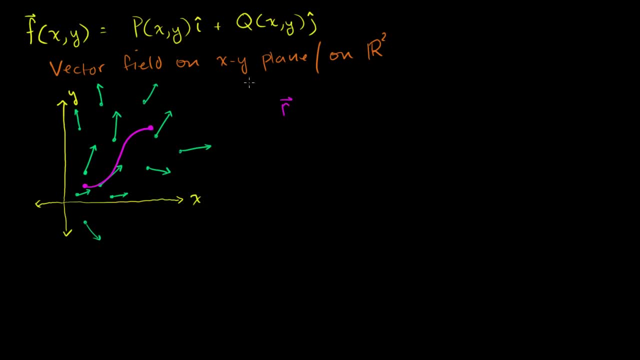 position vector. So let's say that that's defined by r of t, which is just x of t times i, plus y of t times our unit vector j. That's r of t, right there. Well, in order for this to be a finite path, this is true. 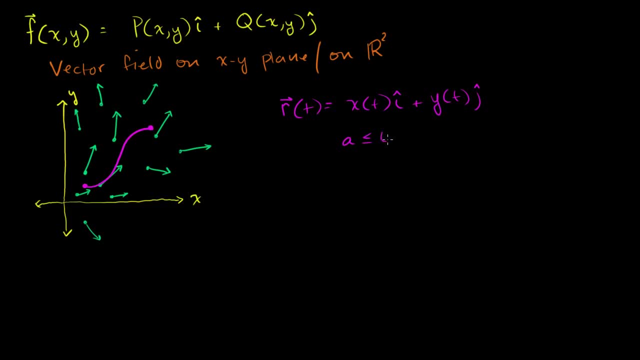 before t is greater than or equal to a and less than or equal to b. This is the path that the particle just happens to take due to all of these wacky forces. So when the particle is right here, maybe the vector field acting on it, maybe it's putting a force like that. 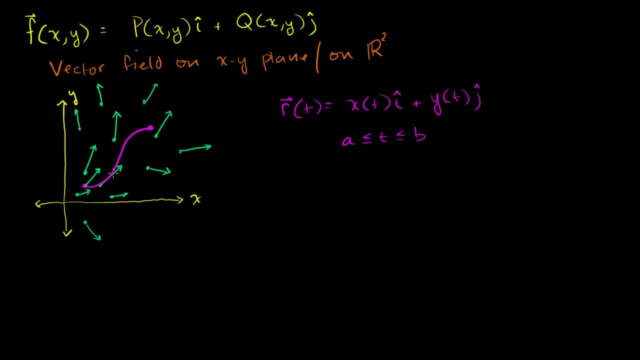 But since the thing is on some type of tracks, it moves in this direction. And then, when it's here, maybe the vector field is like that, but it moves in that direction because it's on some type of tracks. Now, everything I've done in this video is to build up to a 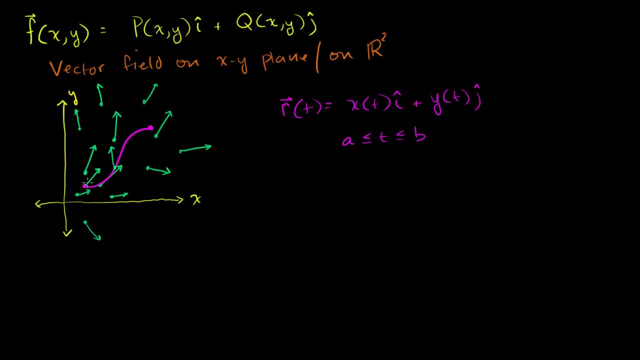 fundamental question: What was the work done on the particle by the field? Work done on the particle, What was the work done on the particle by the field? To answer that question, we could zoom in a little bit. Let's say I'm going to zoom in on only a little small snippet. 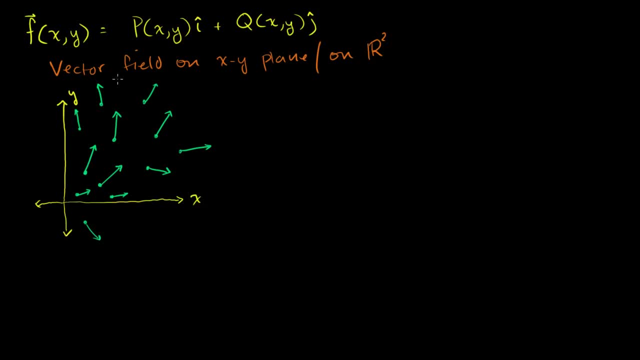 lot of sense that this could be used to describe any type of field. It could be a gravitation field, It could be an electric field, It could be a magnetic field, And this could be essentially telling you how much force there would be on some particle in that field. 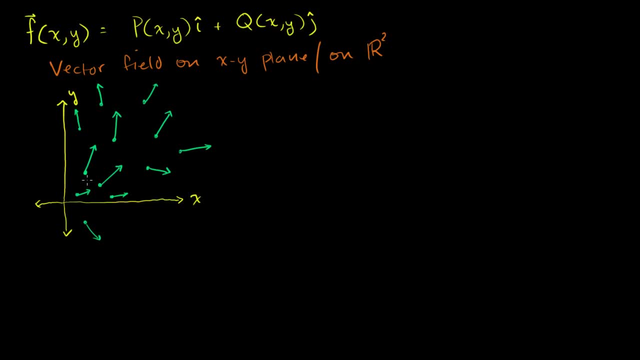 That's exactly what this would describe. Now, let's say that in this field, I have some particle traveling on the xy-plane And let's say it starts here, Let's say it starts there, And by virtue of all of these crazy forces that are acting on, 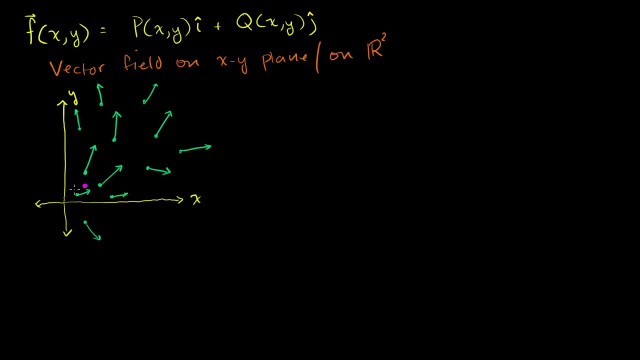 it, and maybe it's on some tracks or something, so it won't always move exactly in the direction that the field is trying to move it at. So let's say it moves in a path that moves something like this, And let's say that this path or this curve is defined by a 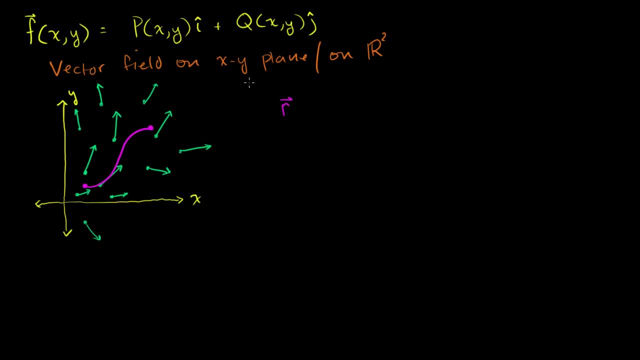 position vector. So let's say that that's defined by r of t, which is just x of t times i, plus y of t times our unit vector j. That's r of t, right there. Well, in order for this to be a finite path, this is true. 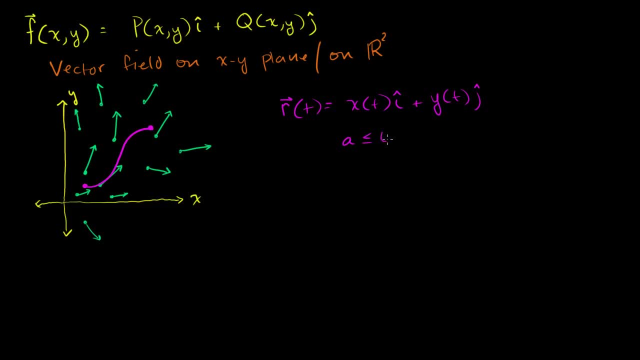 before t is greater than or equal to a and less than or equal to b. This is the path that the particle just happens to take due to all of these wacky functions. So when the particle is right here, maybe the vector field acting on it, maybe it's putting a force like that. 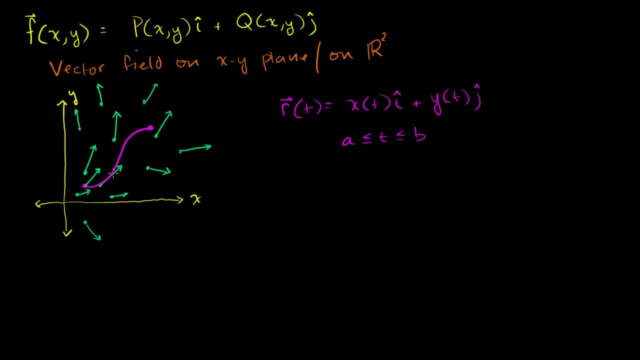 But since the thing is on some type of tracks, it moves in this direction. And then, when it's here, maybe the vector field is like that, but it moves in that direction because it's on some type of tracks. Now, everything I've done in this video is to build up to a 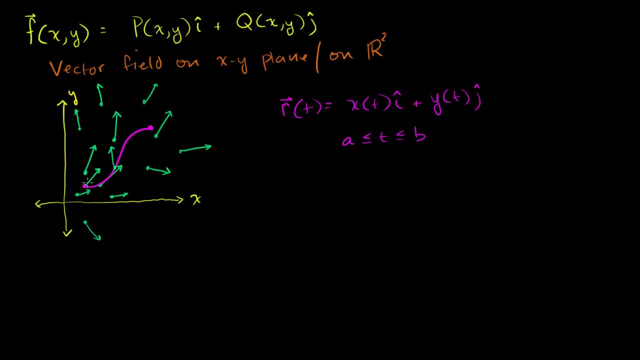 fundamental question: What was the work done on the particle by the field? Work done on the particle, What was the work done on the particle by the field? To answer that question, we could zoom in a little bit. Let's say I'm going to zoom in on only a little small snippet. 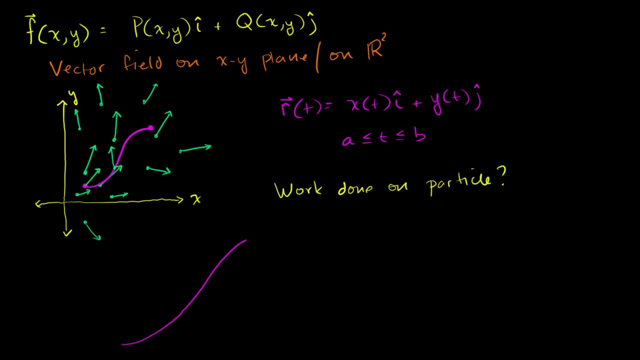 of our path And let's just try to figure out what the work is done in a very small part of our path, Because it's constantly changing. The field is changing directions, My object is changing directions. So let's say when I'm here and let's say I move a small 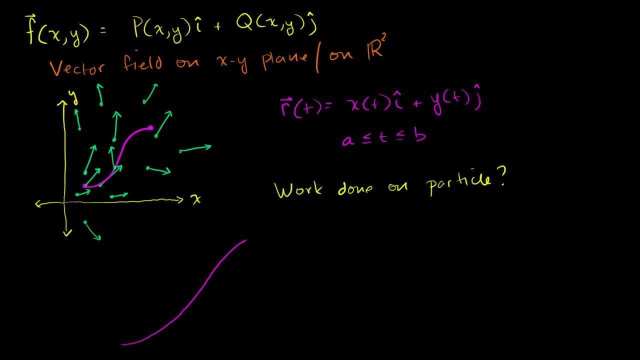 of our path And let's just try to figure out what the work is done in a very small part of our path, Because it's constantly changing. The field is changing directions, My object is changing directions. So let's say when I'm here and let's say I move a small 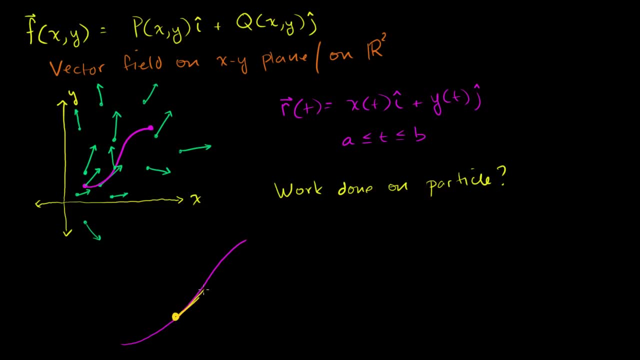 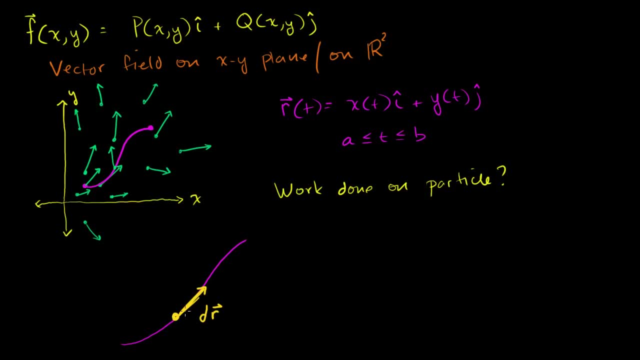 I have a differential vector, infinitely small displacement, And let's say, over the course of that, the vector field is acting in this local area. Let's say it looks something like that, It's providing a force that looks something like that. So that's the vector field in that area, or the force. 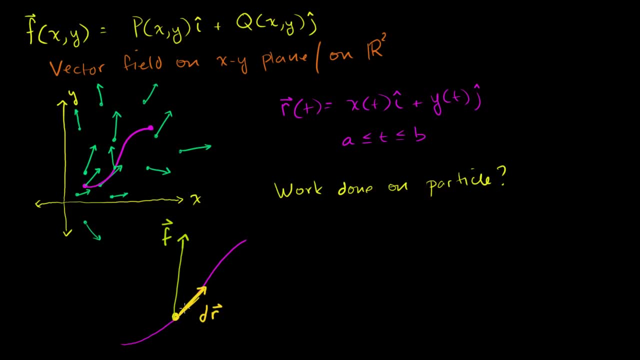 directed on that particle right when it's at that point. This is an infinitesimally small vector. So let's say I move a small amount of time and space, So you could say OK, over that little small point we have. 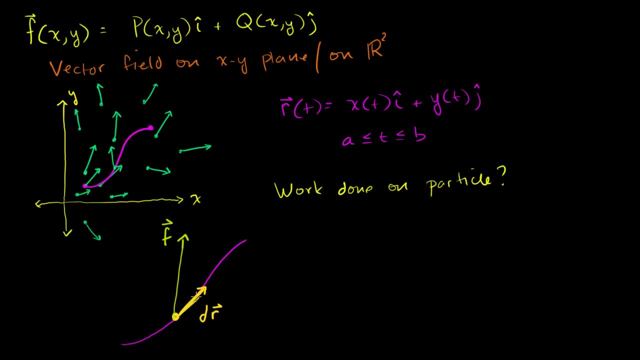 this constant force. What was the work done over this small period? You could say: what's the small interval of work? You could say d work or a differential of work. Well, by the same exact logic that we did with the simple 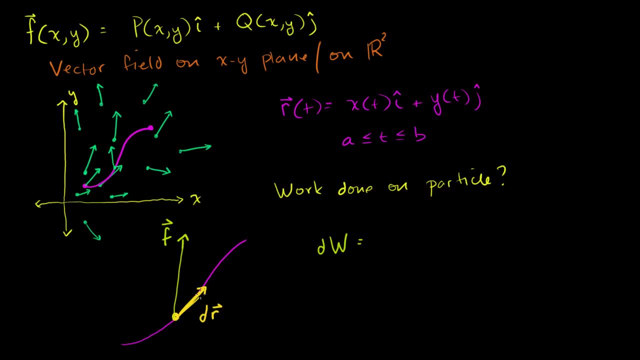 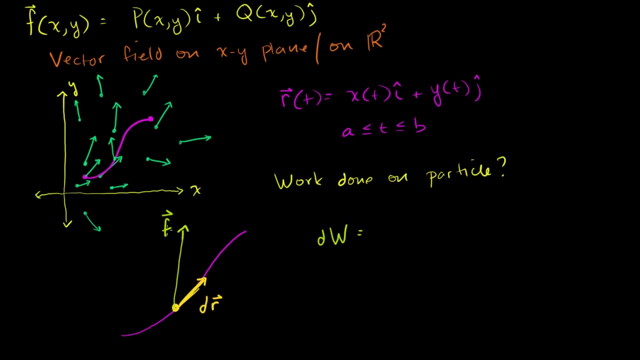 problem. it's the magnitude of the force in the direction of our displacement times, the magnitude of our displacement, And we know what that is just from this example up here. That's the dot product. It's the dot product of the force and our super small 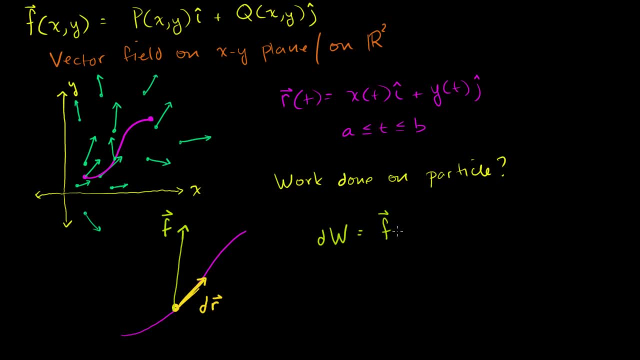 displacement. So that's equal to the dot product of our force and our super small displacement. Now, just by doing this, we're just figuring out the work over, maybe like a really small, super small dr, But what we want to do is we want to sum them all up. 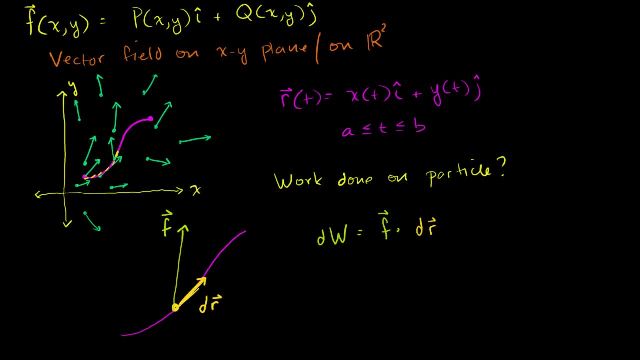 We want to sum up all of the dr's to figure out the total, all of the f dot dr's to figure out the total work done. And that's where the integral comes in. We will do a line integral over. I mean you could think 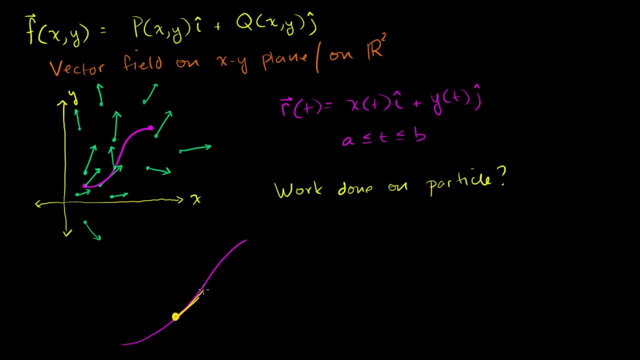 amount of my path. So I'm going to move a small amount of my path. So I'm going to move a small amount of my path. So let's say I move. this is an infinitesimally small dr. I have a differential vector. infinitely small displacement. 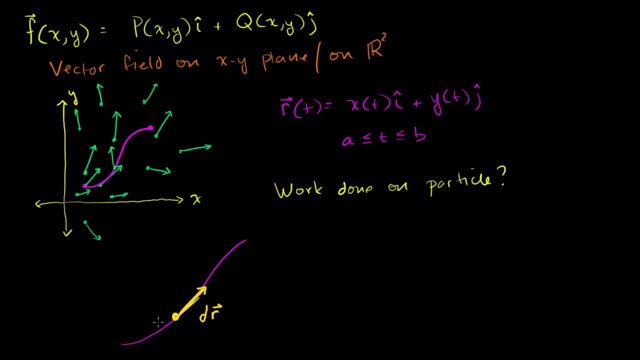 And let's say, over the course of that, the vector field is acting in this local area. Let's say it looks something like that, It's providing a force that looks something like that. So that's the vector field in that area, or the force. 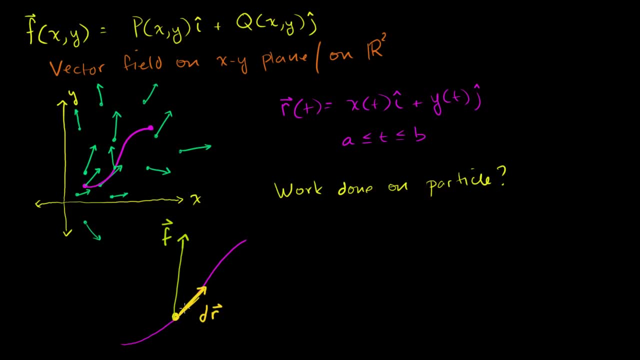 directed on that particle right when it's at that point. This is an infinitesimally small dr. This is an infinitesimally small amount of time and space. You could say OK, over that little, small point we have this constant force. 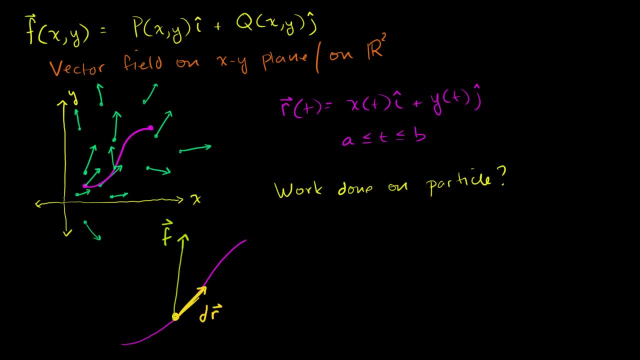 What was the work done over this small period? You could say: what's the small interval of work? You could say d work or a differential of work. Well, by the same exact logic that we did with the simple problem, it's the magnitude of the force in the direction of. 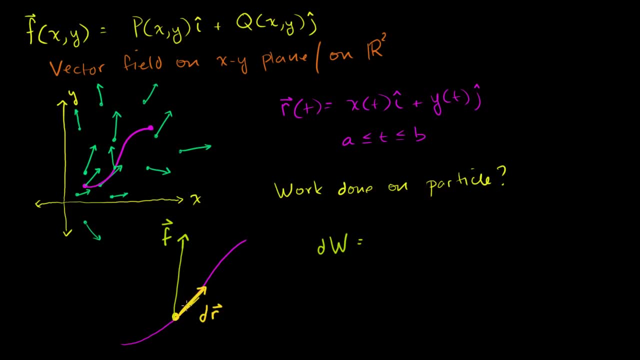 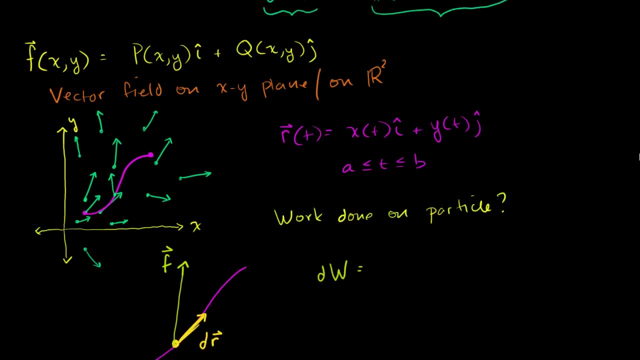 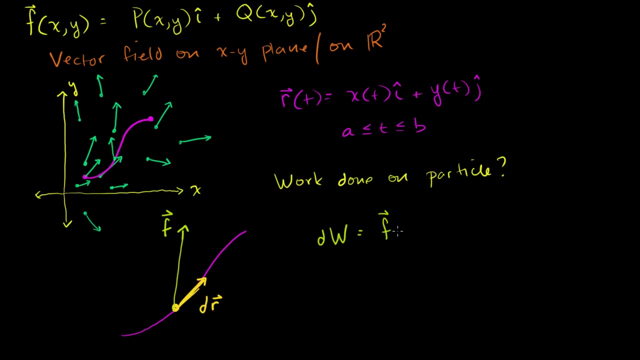 our displacement times, the magnitude of our displacement, And we know what that is, Just from this example up here. That's the dot product. It's the dot product of the force and our super small displacement. So that's equal to the dot product of our force and our. 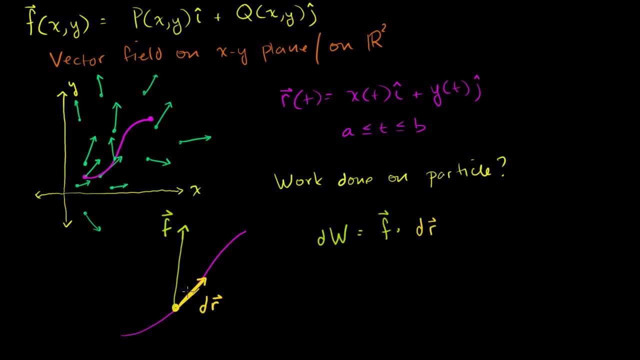 super small displacement. Now, just by doing this, we're just figuring out the work over, maybe like a really small, super small dr, But what we want to do is we want to sum them all up. We want to sum up all of them. 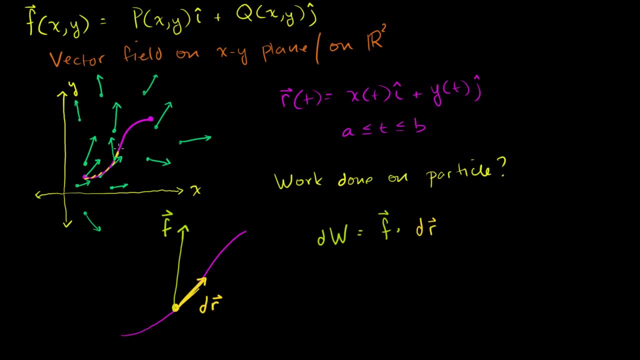 We want to do all of the dr's to figure out the total, all of the f dot dr's to figure out the total work done. And that's where the integral comes in. We will do a line integral over. I mean you could think 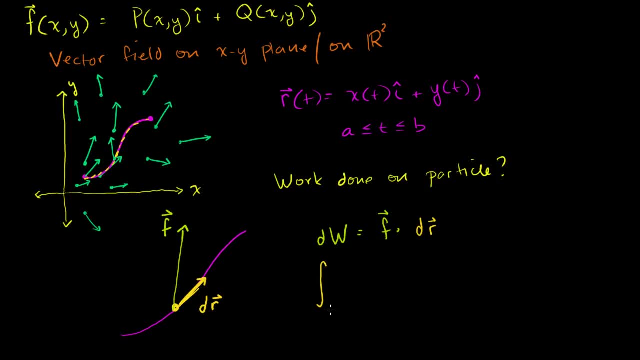 of it two ways. You could write just dw there, but we could say we'll do a line integral that says along this curve c. we could call that c or along r, whatever you want to say it of dw. That'll give us the total work. 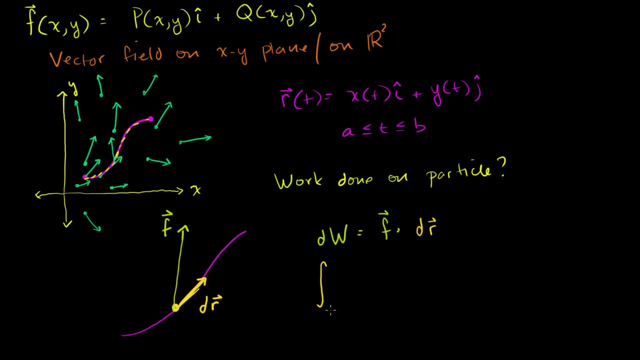 of it two ways. You could write just dw there, But we could say we'll do a line integral that says along this curve c. we could call that c or along r, whatever you want to say it of dw. That'll give us the total work. 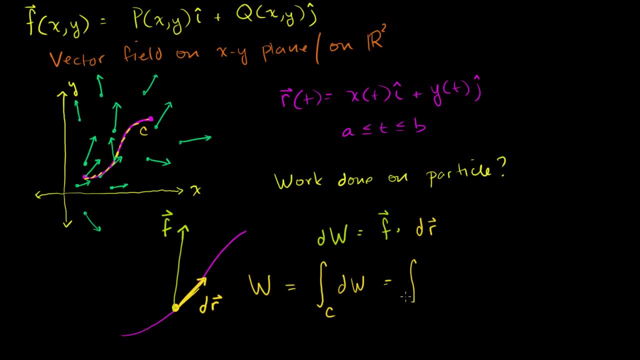 So let's say work is equal to that. Or we could also write it over the integral, over the same curve of f, dot, dr, And this might seem like a really gee. this is really abstract, Sal. How do we actually calculate something like this? 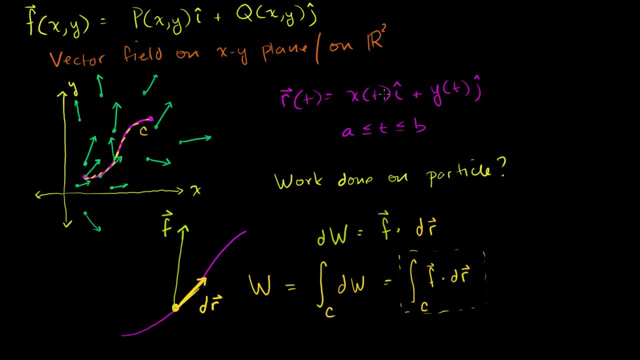 Especially because we have everything parametrized in terms of t. How do we get this in terms of t? And, if you just think about it, what is f dot r Or what is f dot dr? Well, actually, to answer that, let's think about, let's. 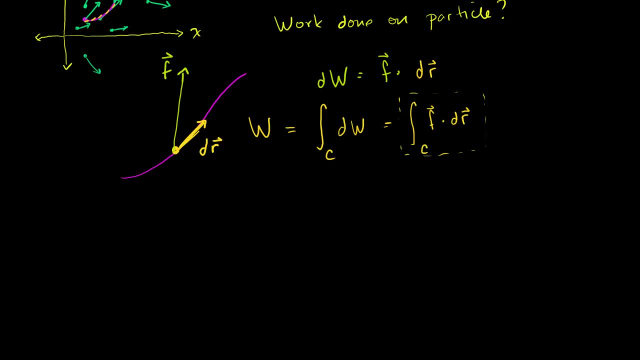 remember what dr looked like. If you remember, dr dt is equal to x prime of t. I'm writing it like I could have written dx dt if I wanted to times the i unit vector plus y prime of t times the j unit vector. 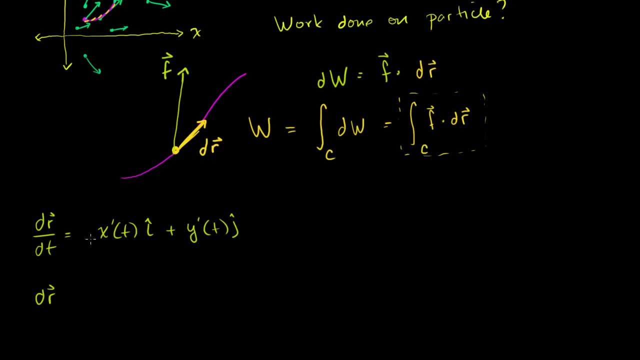 And if we just wanted dr, we could multiply both sides. if we're being careful, We're being a little bit maybe more hand-wavy with the differentials, not too rigorous We'll get. dr is equal to x prime of t dt times the unit. 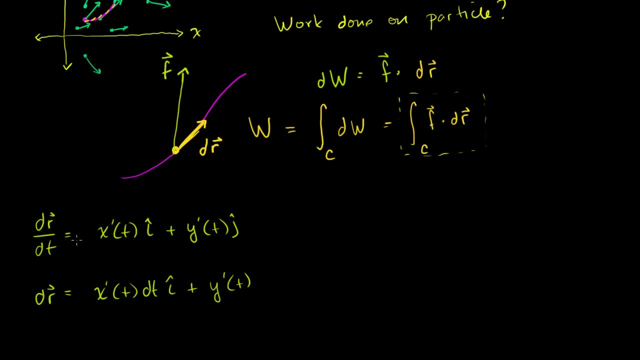 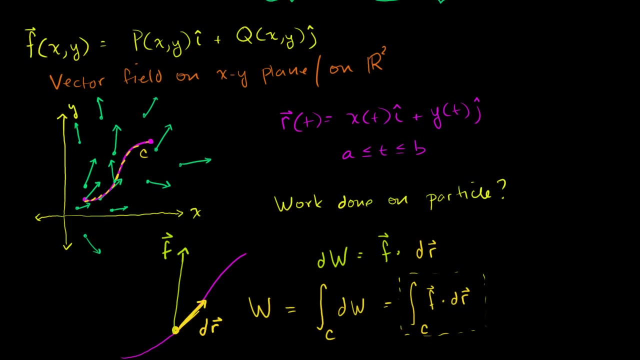 vector i plus y prime of t times the differential dt times the unit vector j. So this is our dr, right here. That is our dr, And remember what our vector field was? It was this thing up here. Let me copy and paste it. 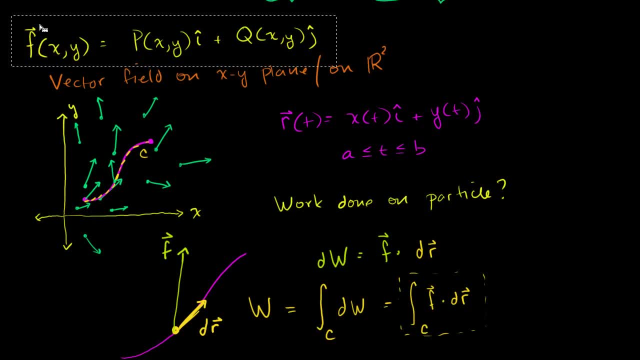 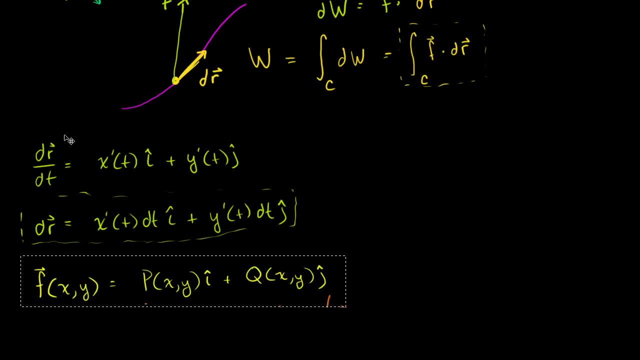 And then we'll see that the dot product is actually not so crazy. So I'm going to copy and then let me paste it down here. All right, I'll paste it down there. So what's this integral going to look like? This integral right here, that seems- gives us the total work. 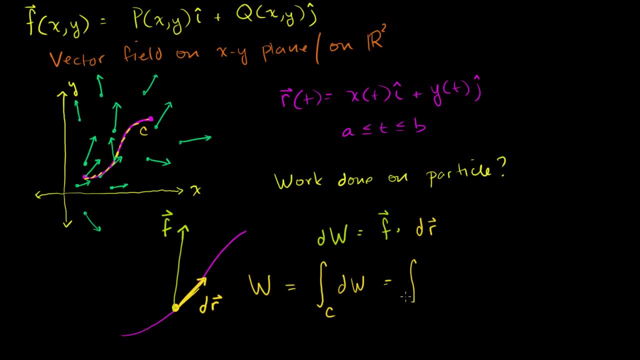 So let's say work is equal to that. Or we could also write it over the integral, over the same curve of f, dot, dr, And this might seem like a really gee. this is really abstract, Sal. How do we actually calculate something like this? 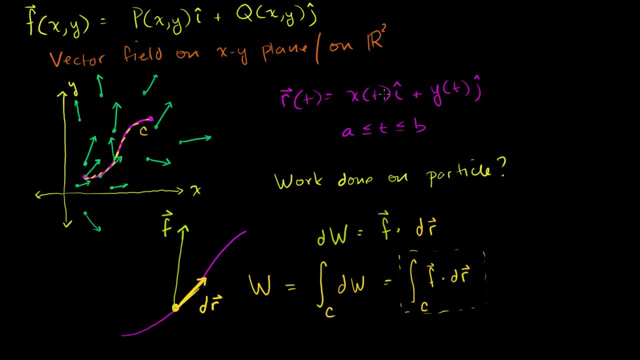 Especially because we have everything parametrized in terms of t. How do we get this in terms of t? And, if you just think about it, what is f dot r Or what is f dot dr? Well, actually, to answer that, let's think about, let's. 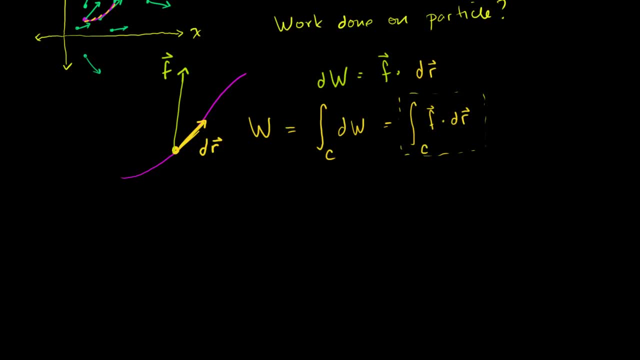 remember what dr looked like. If you remember, dr dt is equal to x prime of t. I'm writing it like I could have written dx dt if I wanted to times the i unit vector plus y prime of t, times the j. 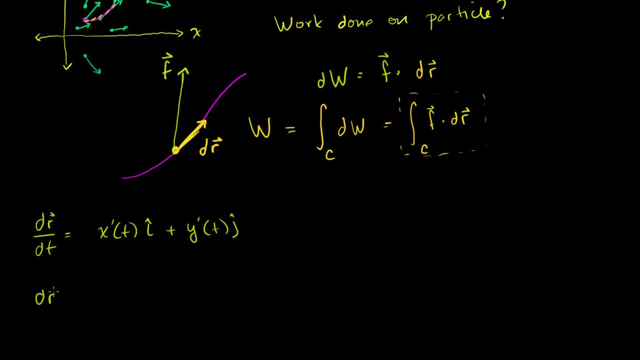 unit vector. And if we just wanted dr, we could multiply both sides. if we're being careful, We're being a little bit maybe more hand-wavy with the differentials, not too rigorous We'll get. dr is equal to x prime of t dt times the unit. 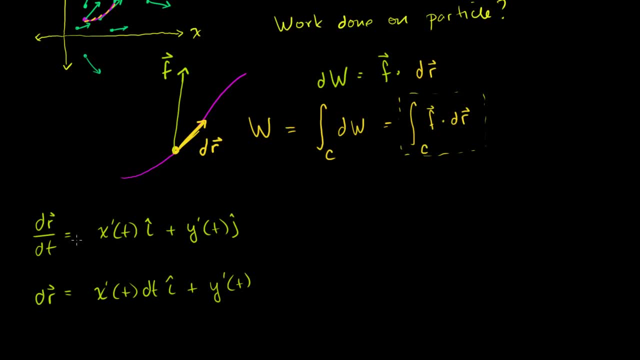 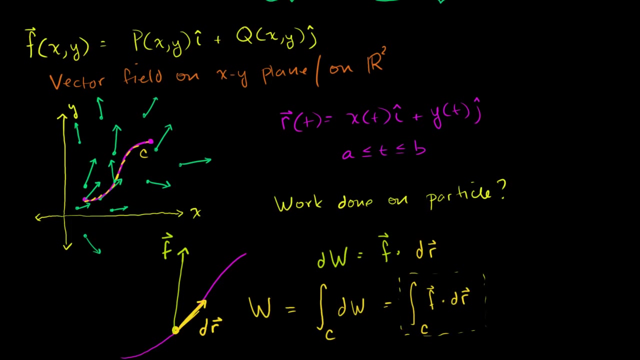 vector i plus y prime of t times the differential dt times the unit vector j. So this is our dr, right here. That is our dr, And remember what our vector field was? It was this thing up here. Let me copy and paste it. 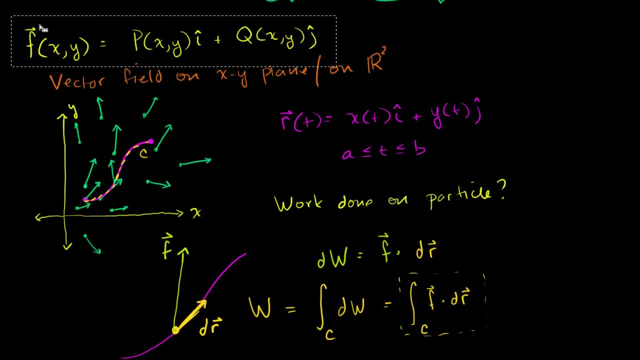 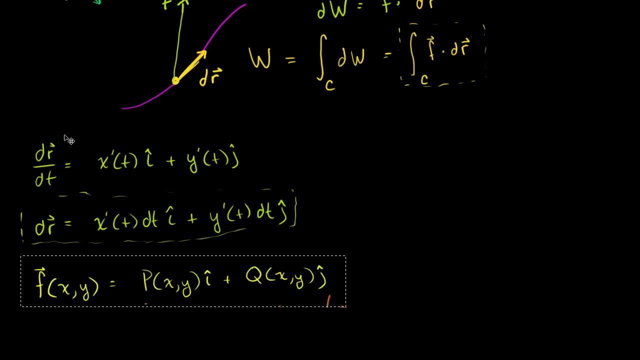 And then we'll see that the dot product is actually not so crazy. So I'm going to copy and then let me paste it down here. All right, I'll paste it down there. So what's this integral going to look like? This integral right here, that seems- gives us the total work. 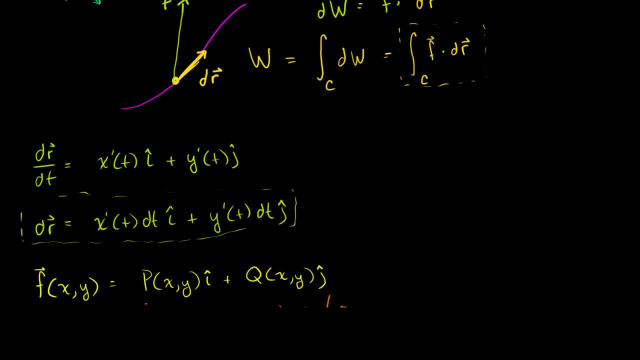 done by the field on the particle as it moves along that path, which is super fundamental to pretty much any serious physics that you might eventually find yourself doing. So you could say: well, gee, it's going to be the integral. well, let's just say: from t is equal to a to t is equal to b.